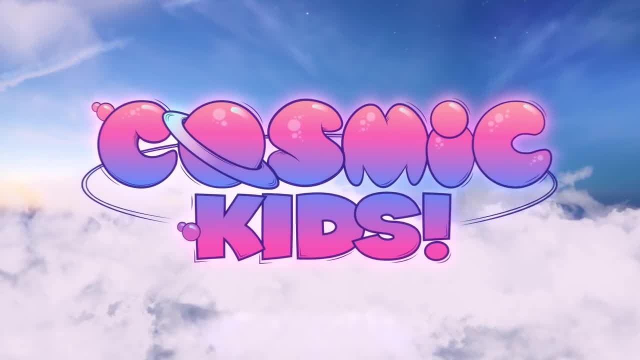 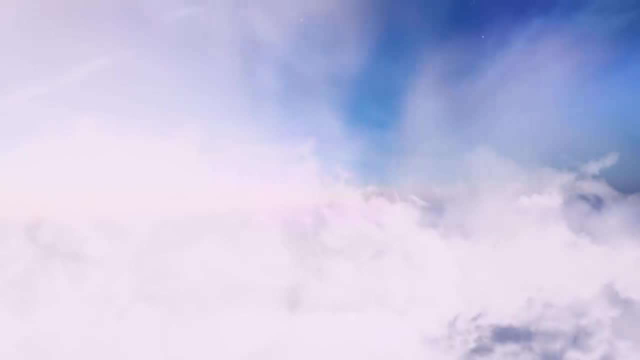 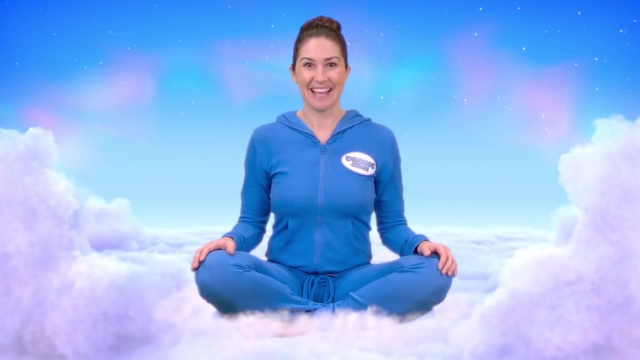 Hello everyone. welcome to the Cosmic Kids Zen Den, your place to feel all calm and relaxed and to help our minds stay healthy and happy. First let's get comfy. Sitting on our bottoms with our legs crossed, we take two nice deep breaths In through our nose and out through 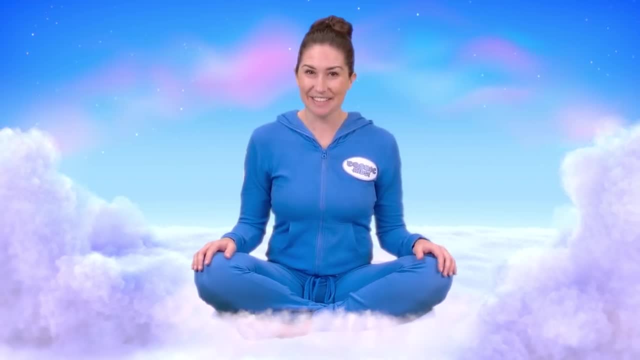 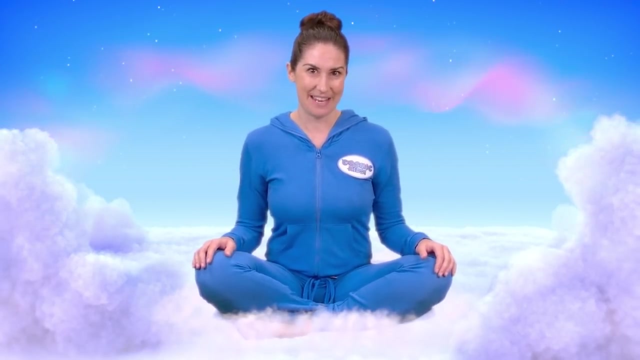 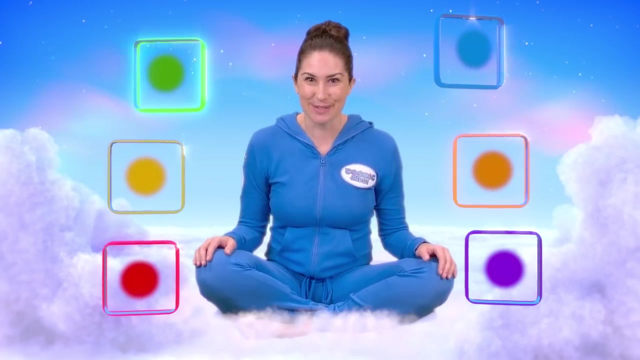 our mouth And again in through our nose and out through our mouth. Now let's get the Zen Den ready so we can really enjoy it. Let's fill it with colour. Wow, Lots of great colours to choose from. Let's pick one that helps us feel all lovely. 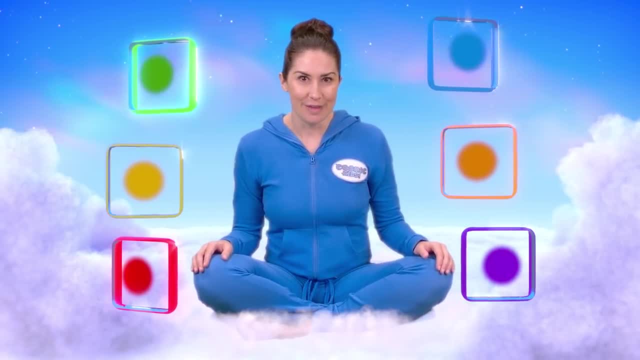 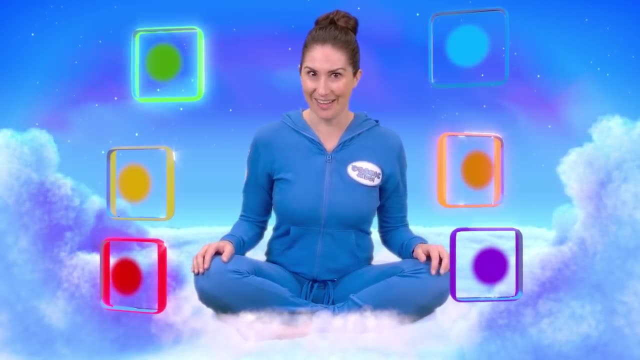 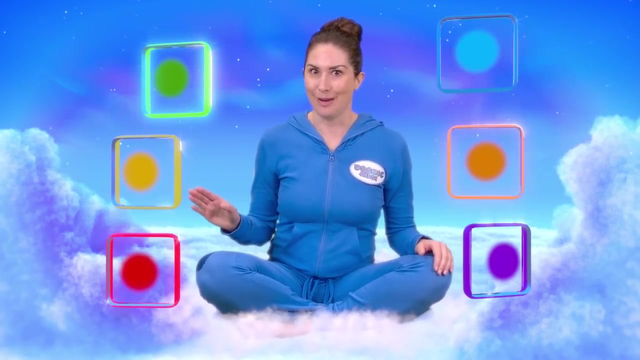 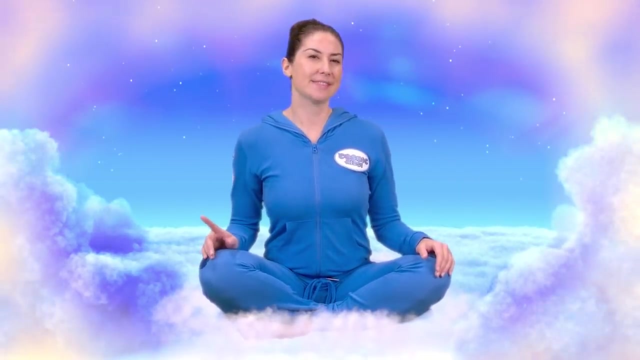 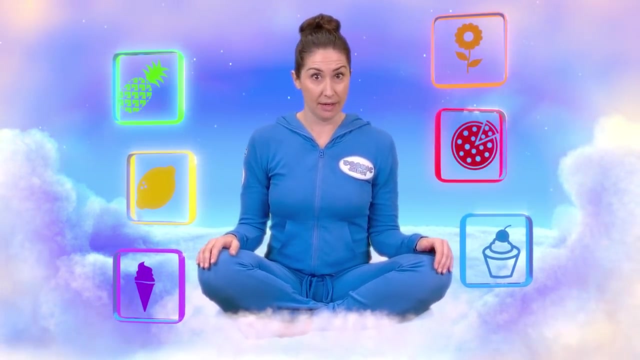 and calm. This lovely blue looks good. Let's have that. And what about a no colour? Shall we have one more? Okay, let's add this sunny yellow colour. That's it Now for the smell. These look interesting. Pineapple smell, Pizza smell. 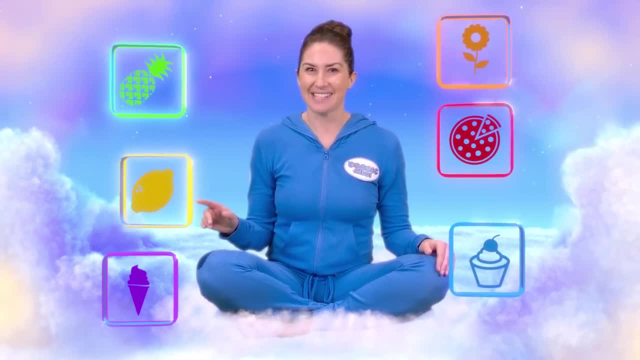 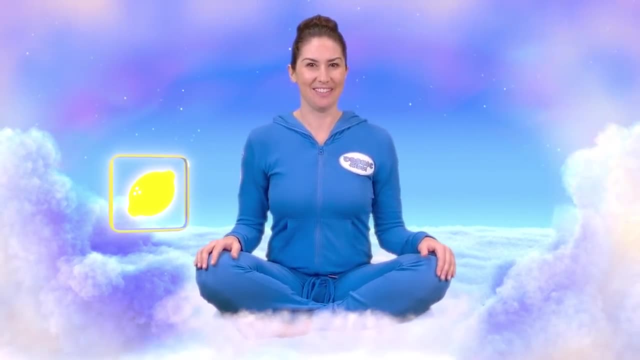 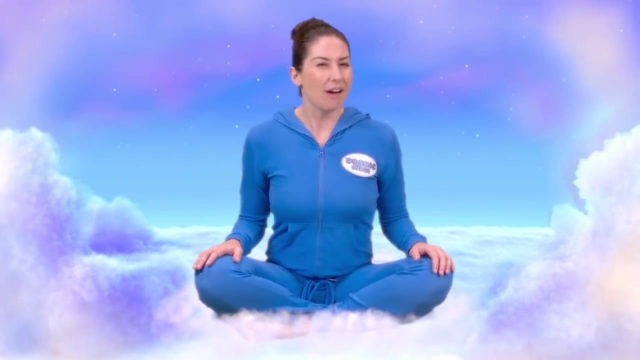 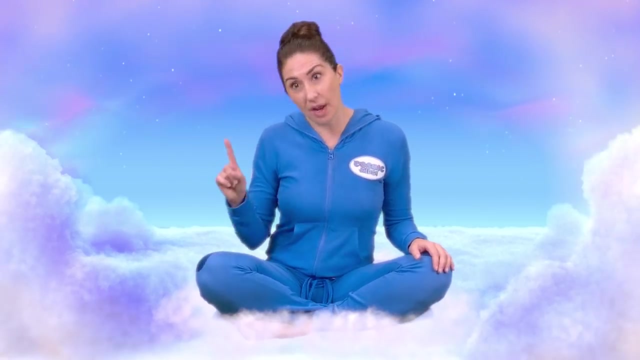 Mmm. Ah, yes, let's smell the lemon, Mmm. lemon is a good, bright smell and helps us concentrate. Now here's a question for you. On a scale of 1 to 10, how good do you think you are at listening, With 1 not being very good and 10 being the? 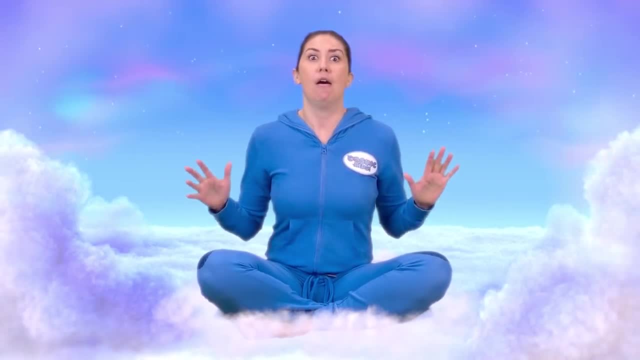 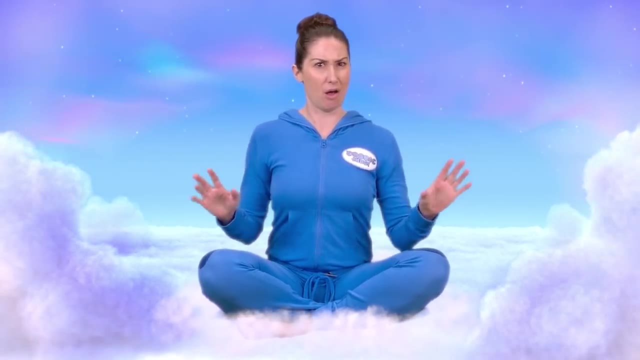 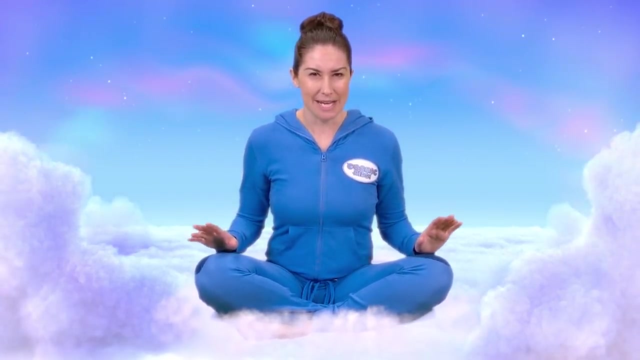 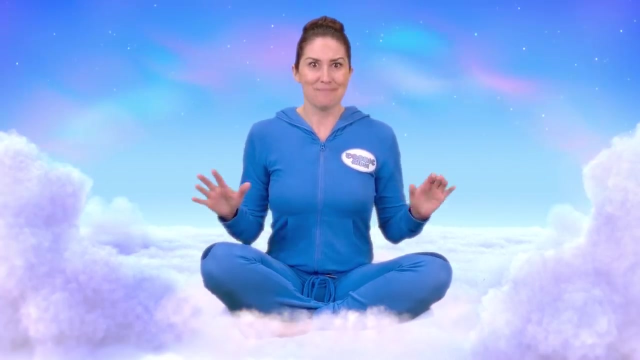 best in the world. Okay, so lots of you reckon you're pretty good, some not so much, and some are the masters of listening. Well, if you're that good, maybe you're really Spider-Man. Have you heard about Spidey senses? Hmm, Well, let's now play a special game to see how. 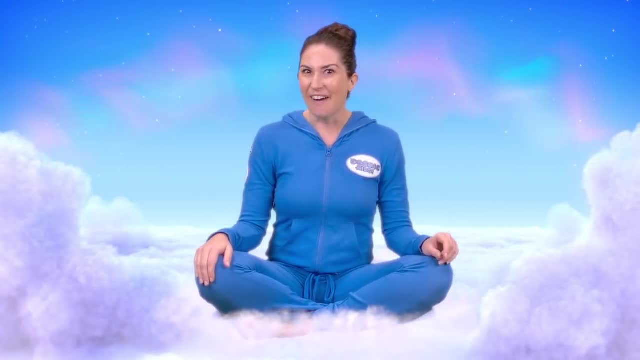 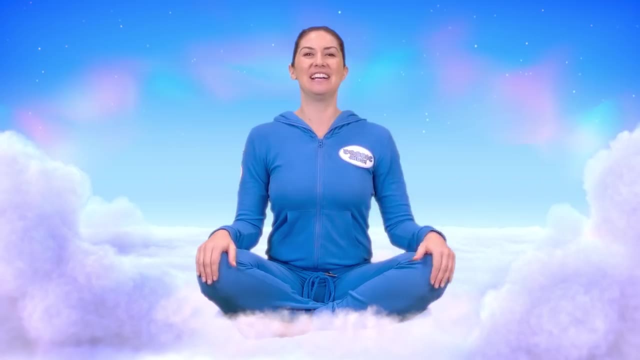 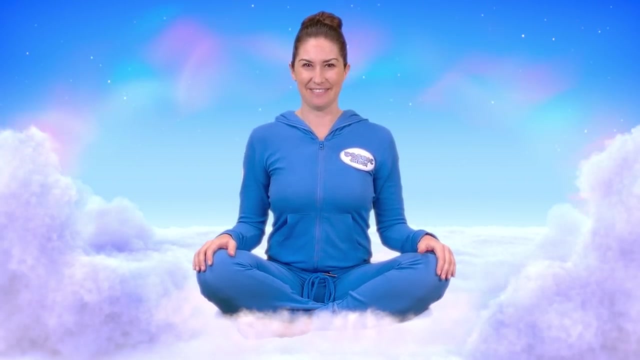 good we are at listening and how strong our senses are- Spidey senses are. It's time to activate our listening. So keep your hands resting on your knees, Make your back long and strong, so you are switched on and ready. Now listen, for when you hear the bell, The sound will then fade until it's gone. 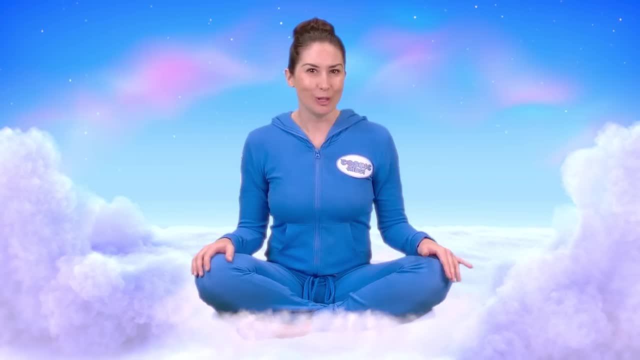 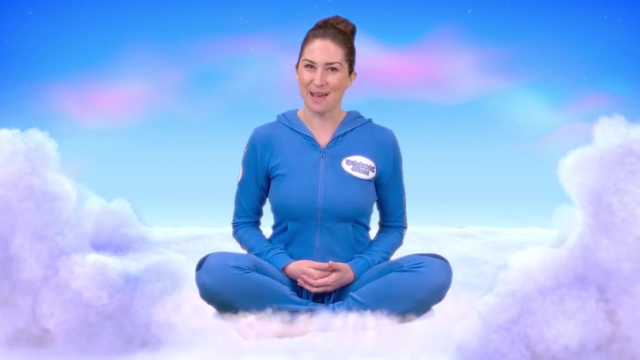 I want to see how long you can hear the sound of the bell ringing And when you can't hear it any longer, move your hands from your knees into your lap. Then I'll be able to see how long you could hear the bell and how good your listening was. Ready, Let's take our 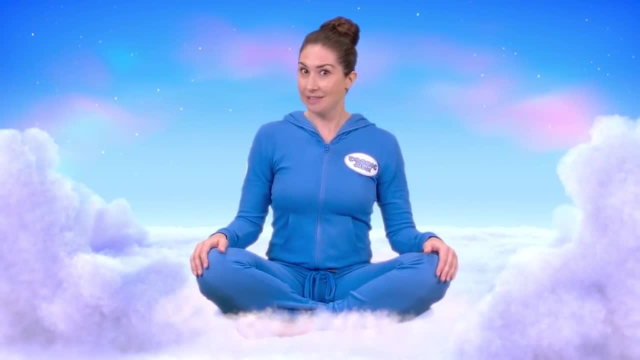 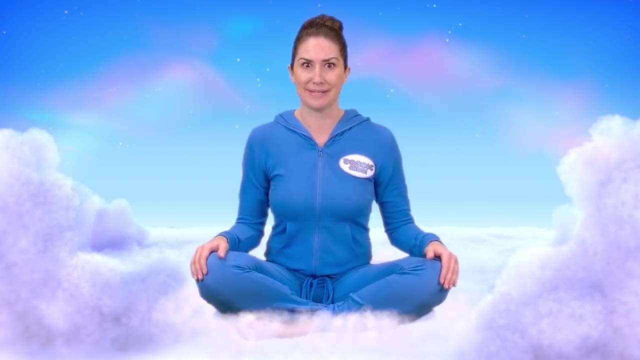 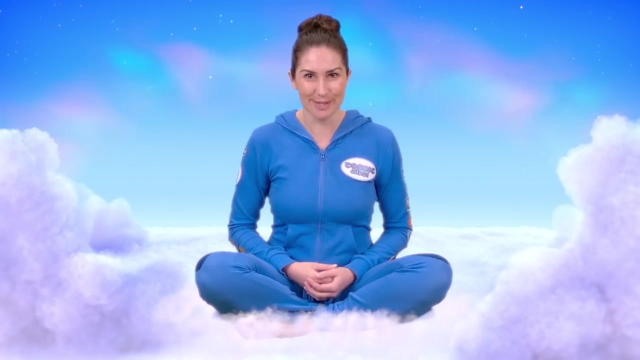 hands onto our knees And, if you want, you can put your hands on your knees, and if you want, you can also close your eyes, so you're totally focused on your listening. So here comes the sound of the bell. Well, that was a good start. You're already showing. 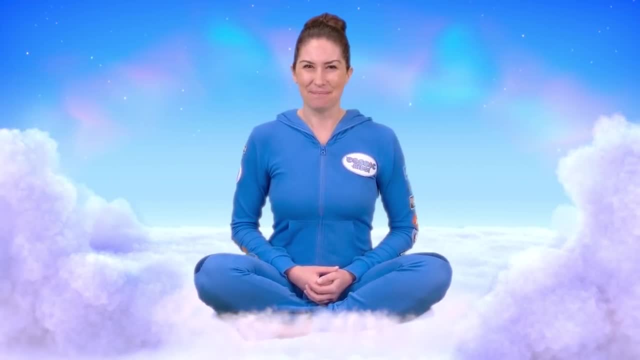 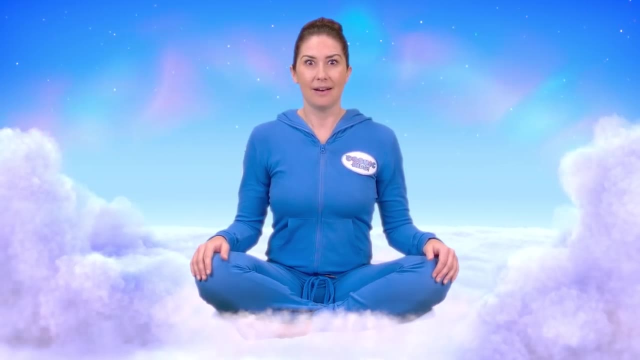 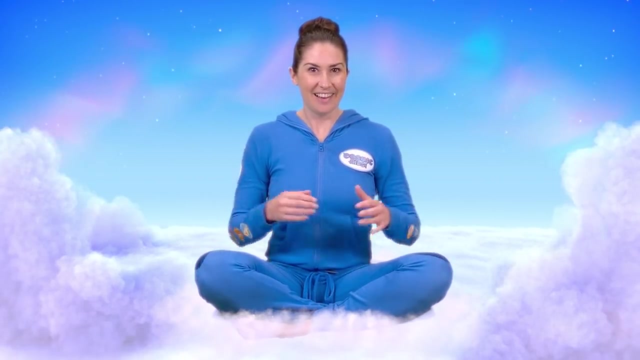 how good you are at listening. Let's try it again. Ready Hands back to knees- Cool, That was even better than the first time. Great listening everyone. Let's do one more, one last time to see if we can stretch those Spidey senses. 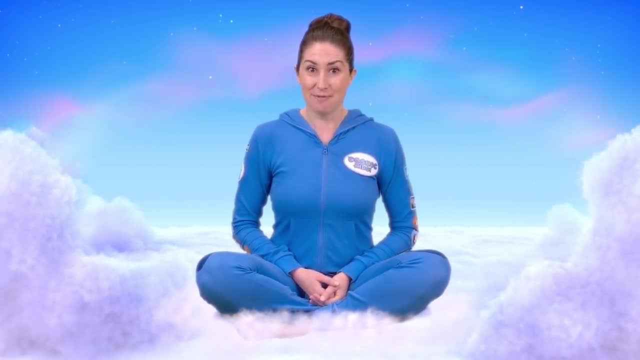 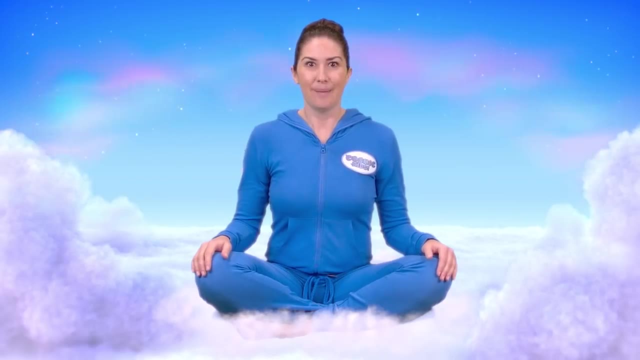 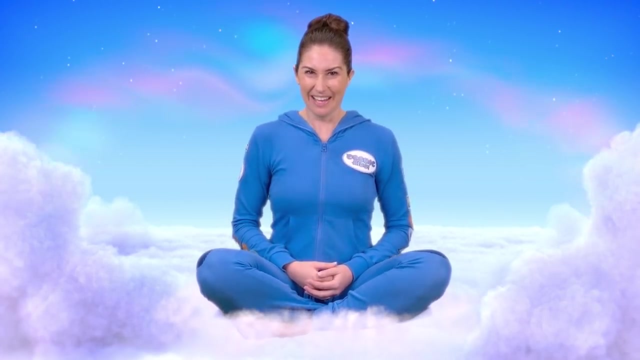 Wow, that was the best one. Now you've proven just how great your listening skills can be. Your spider sense is activated. Next time you are trying to learn something from the teacher or someone is telling you something, see if you can activate your listening as.